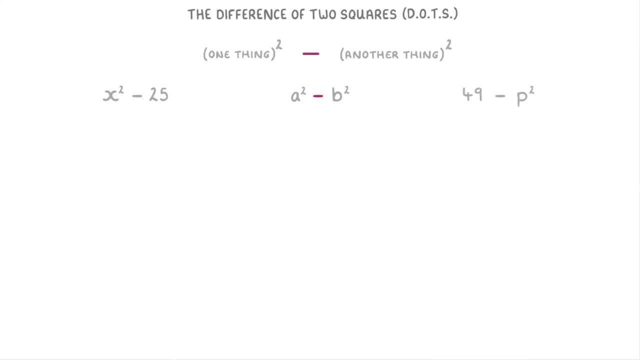 squared minus 25, or 49 minus p squared. To factorize these expressions, all you need to do is figure out the two things that are being squared. So in our a squared minus b squared example, that would be a and b. And then we stick these into two sets of brackets, one where we add them. 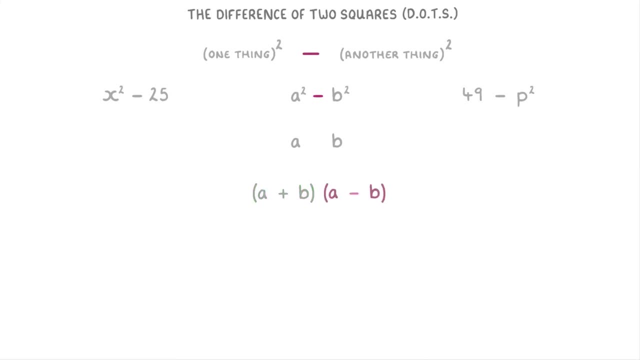 together, so a plus b, and the other where we subtract them, so a minus b, And it's always the second thing that you subtract from the first. Now this rule by itself might not make much sense, so let's have a go at these two questions now and see how it actually works In this. 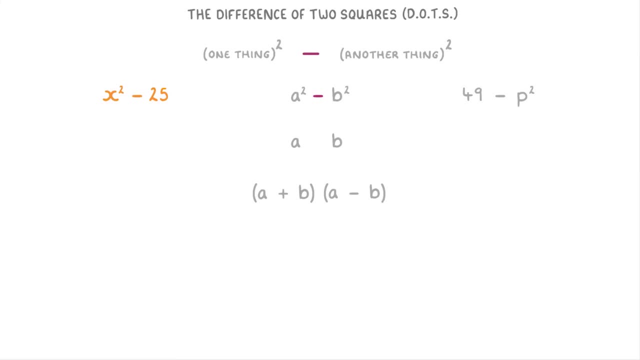 first one. we're trying to factorize x squared minus 25.. So the first thing we need to do is figure out what it is that's being squared to get each of these two terms For x squared. it's easy to spot that it's an x being squared, so we can write that below, Although another way to think. 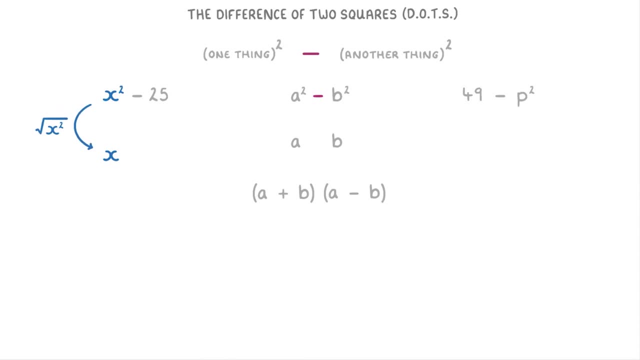 about it is that we're just finding the square root of x squared, which is x. Then, if we do the same thing over and over again, we'll be able to find the square root of x squared. So we write that below as well. Then all we have to do is put these numbers into two sets of brackets: one where we 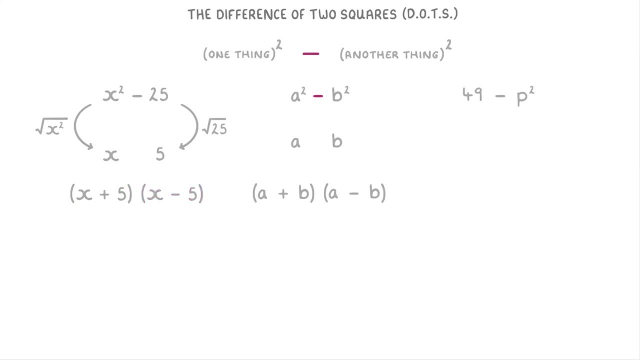 add them together, so x plus 5, and one where we subtract them, so x minus 5.. Next up, we have 49 minus p squared. So in this case we need to notice that 49 is just 7 being squared and that p squared. 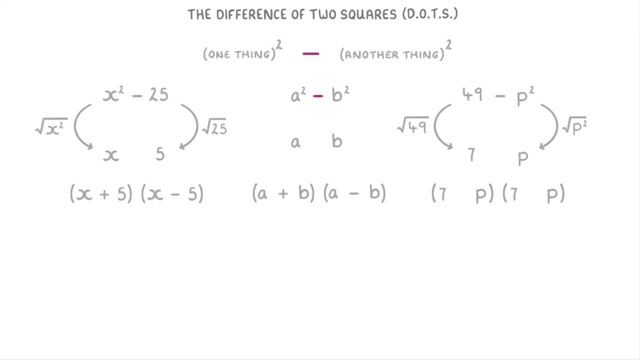 is being squared, So we put the 7 and the p into our brackets as 7 plus p and 7 minus p. Let's have a go at these two slightly harder ones now. This first one, 16 x squared minus 9 y squared, is a little bit different to the ones we've seen, so 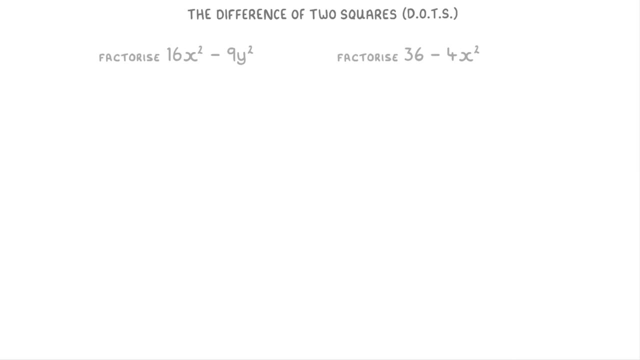 far, because the two terms contain numbers and letters. this time. The way we work it out, though, is exactly the same, but we're going to have to find the square root of x squared, So we're going to do the same. So the first step is to find the square root of each term, The square root of 16 x. 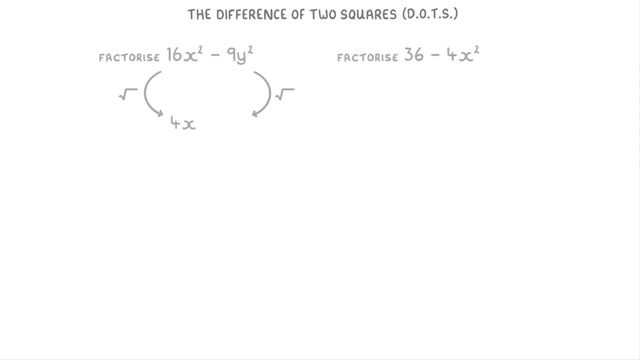 squared is just 4x, because the square root of 16 is 4, and the square root of x squared is x. The same thing works for 9. y squared Its square root is 3y, because the root of 9 is 3, and the root of y squared is y. 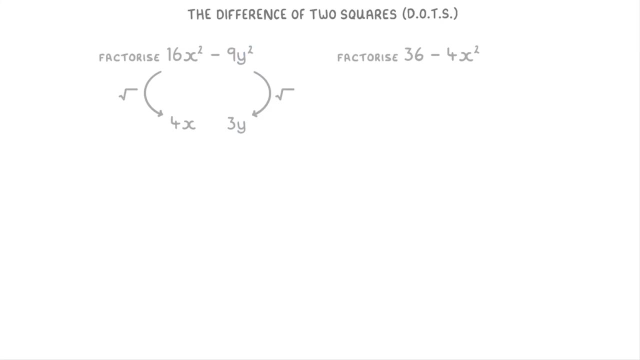 So all that's left is to put 4x and 3y into the two sets of brackets, So 4x plus 3y in the first and 4x minus 3y in the second. In this next one we need to factorize 36 minus 4x squared. So because the square root of 36 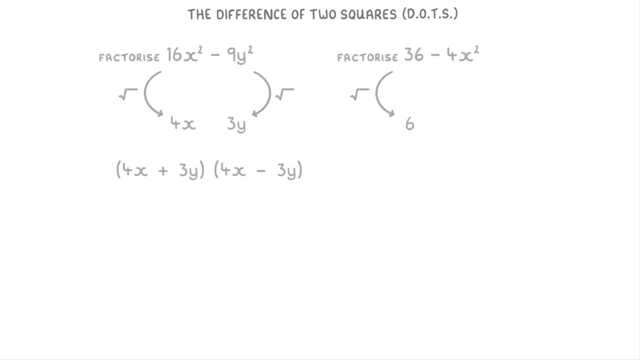 is 6, and the square root of 4x squared is 2x, our brackets will be 6 plus 2x and 6 minus 2x. Let's try two more to finish. In this first one we're trying to do 9x squared minus 64.. 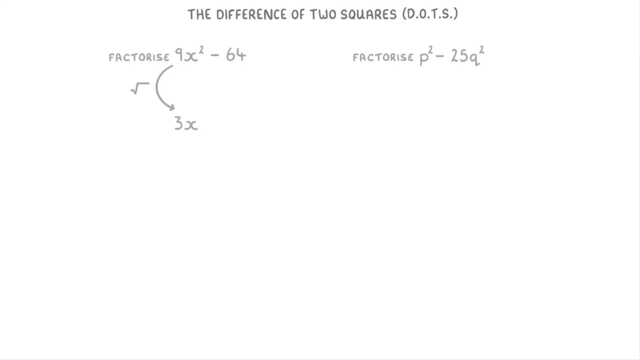 So we can square root the 9x squared to get 3x and square root the 64 to get 8.. Meaning we get the brackets 3x plus 8, and 3x minus 8.. For this last one, p squared minus 25q squared, the square root of p squared is p. 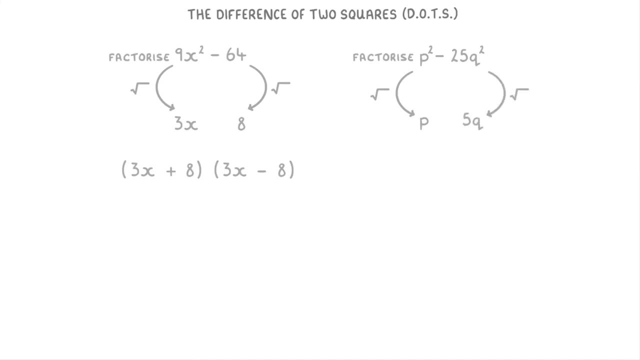 and the square root of 25q squared is 5q, So we get p plus 5q and p minus 5q. Before we finish, I just want to show you that this technique of factorizing really does work, which we can do by expanding the brackets back out and double checking that there is a